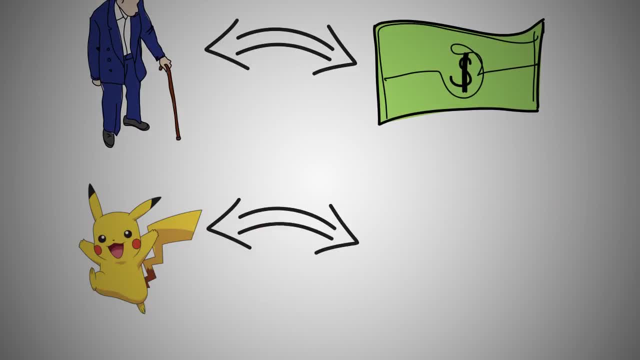 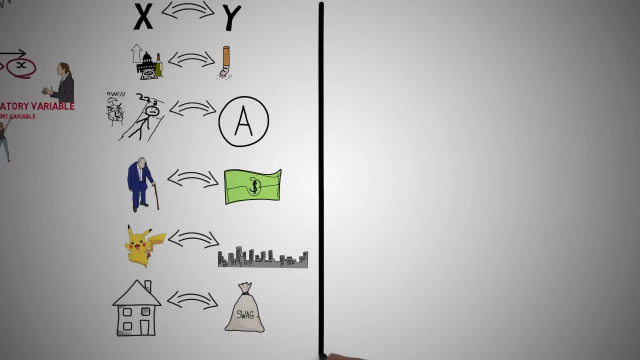 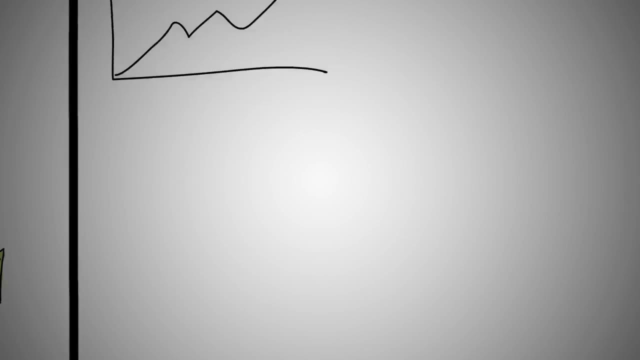 experience versus salaries, pokemon versus urban density and house floor area versus house price. The second application is to forecast new observations. we can use what we already know to forecast unobserved values. here are some examples of the way linear regression can be applied. so say, the return on investment of fidget spinners over time, as well as stock. 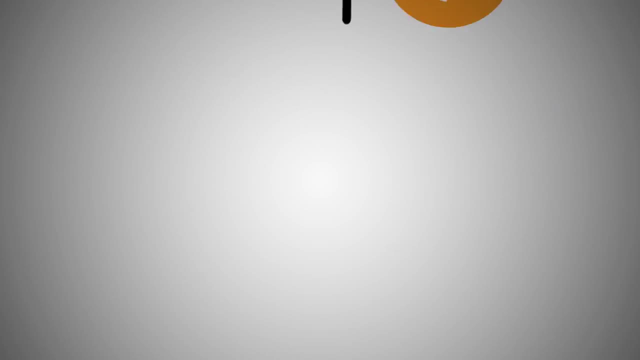 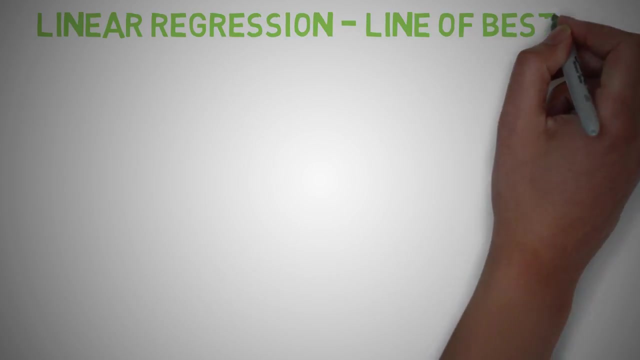 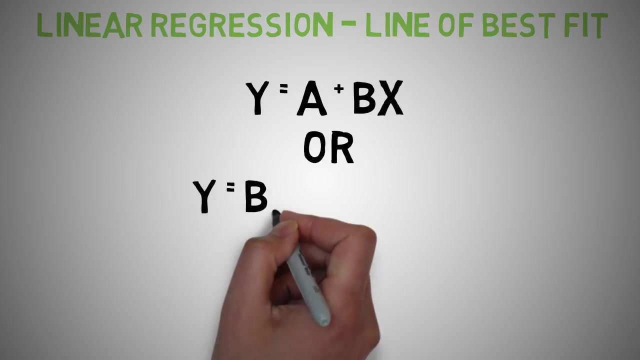 price over time, or to predict the price of bitcoin over time. So you can think of linear regression as the line of best fit. So the line of best fit can be represented by the linear equation: y equals a plus bx, or y equals mx plus b, or y equals b0 plus b0.. 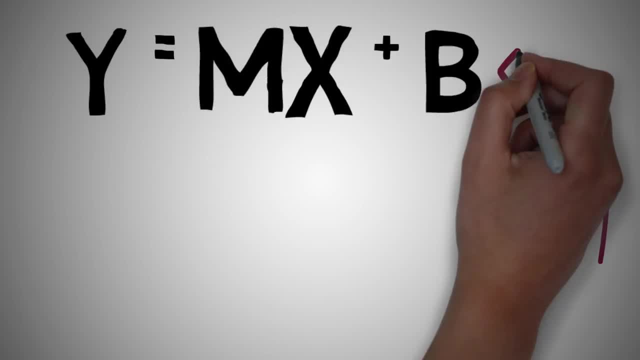 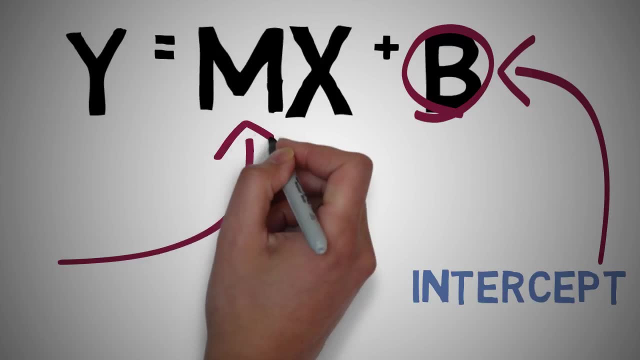 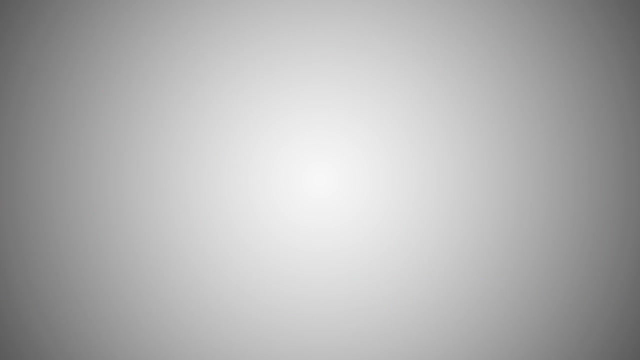 You mostly learned this in school. So b is the intercept. if you increase this variable, the intercept moves up or down along the y-axis, And m is the slope or gradient. if you change this, then your line rotates along the intercept. 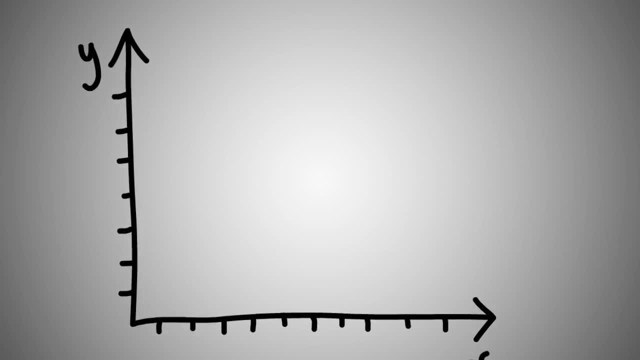 So data is actually a series of x and y observations, as shown on the scatter plot. They don't follow a straight line. however, they do follow a linear pattern, hence the term linear regression. Assuming that we already have the best fit line, we can calculate the error term epsilon. 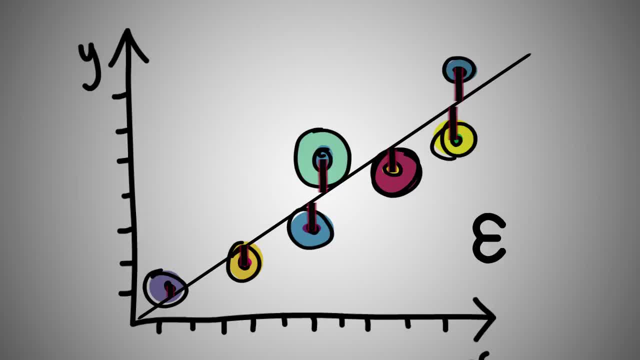 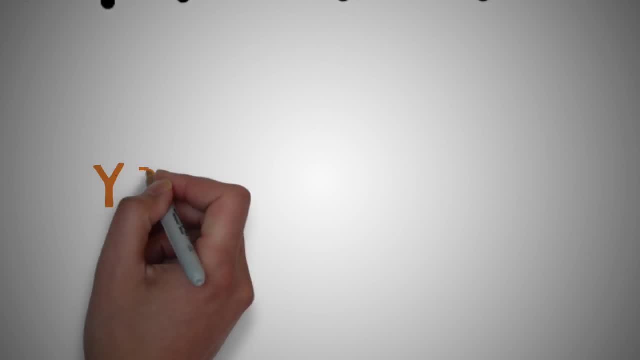 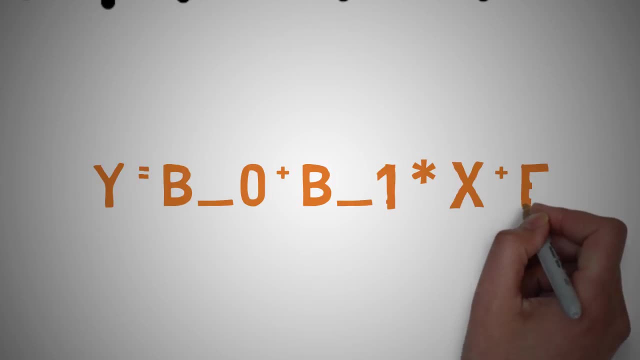 also known as the residual, And this is the term that we would like to minimize along all the points in the data series. So say, we have our linear equation represented in statistical notation. the residual fits into our equation as shown. y equals b0 plus b1 times x plus epsilon. 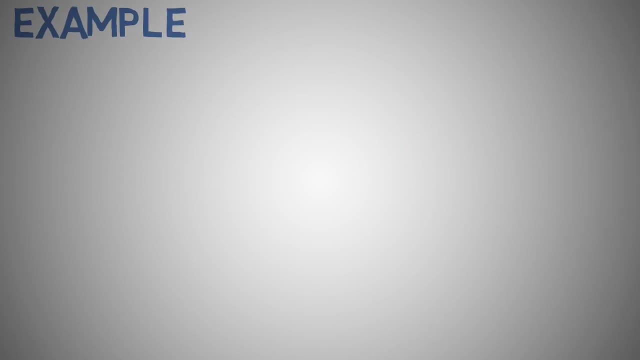 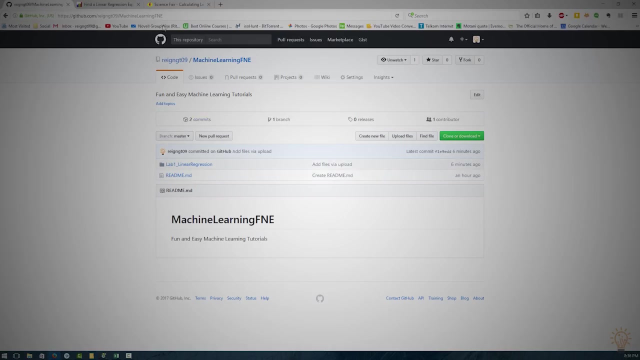 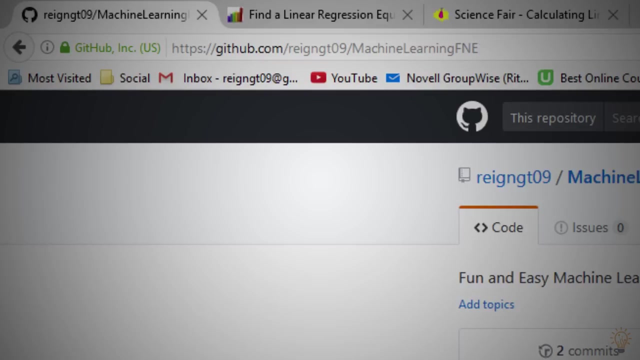 Okay, let's try doing this by hand In an example. Okay, so over here we have our dataset of pokemon versus urban density, And this dataset you can get from my github repository on the range et09 and machine learning, fne, which stands for fun and easy. 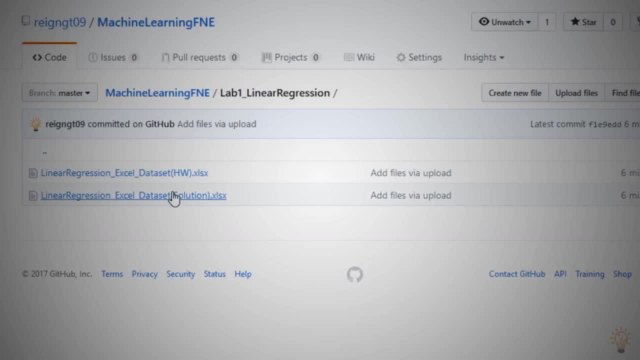 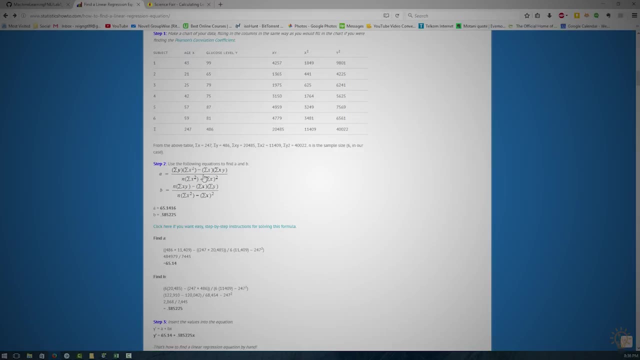 Go to lab1, linear regression, and then you will have the homework package that you can work on, and then, as well as the solution, Over here on this site, you will be able to find the same dataset, as well as the equations defining the coefficients of a and b. 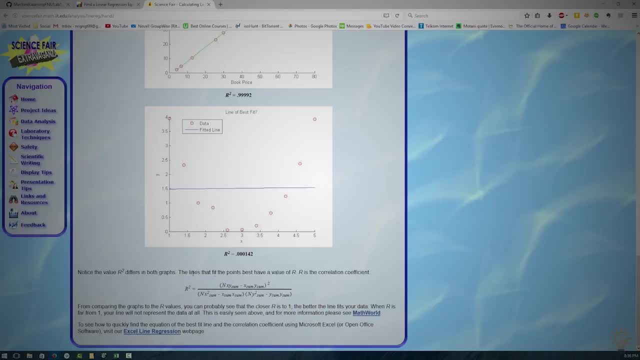 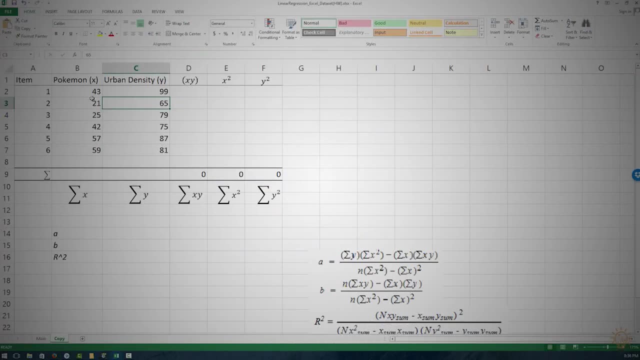 And then to find the correlation coefficient squared. you can find that equation right over here And you can just follow the address. Okay, so we have pokemon, which is on our x-axis, our y-axis is urban density, and then we can create a plot, a scatter plot, of that. 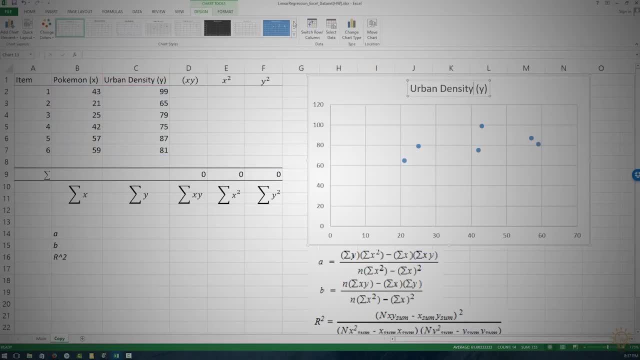 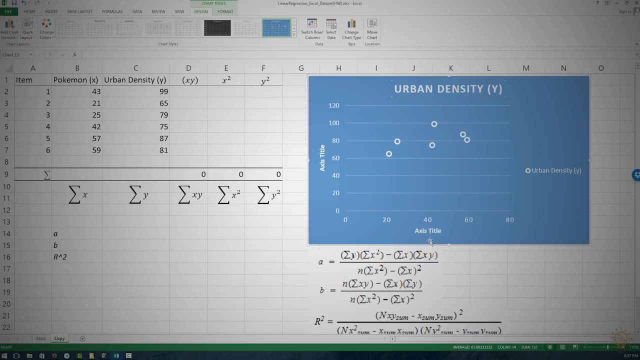 And then we can just format it to make it look a little bit nice. Okay, Let's add in some data labels And then we're going to be calling this urban density on the y-axis And then we're going to label this axis pokemon quantity. 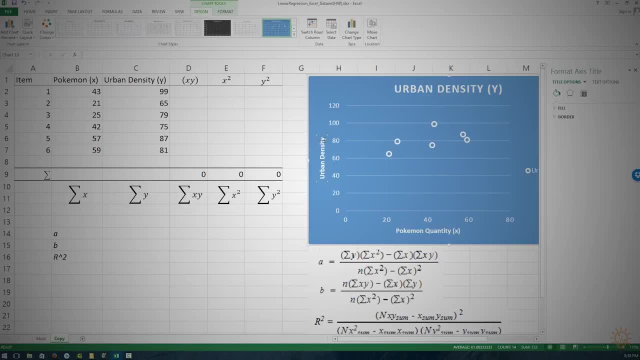 Now, remember, this is just a mock dataset. You can fill it with any data that you want, Or you can import a legitimate dataset. Okay, so this is the equation that we get from our trend line, And we're going to create it on our own and calculate the coefficients by hand. 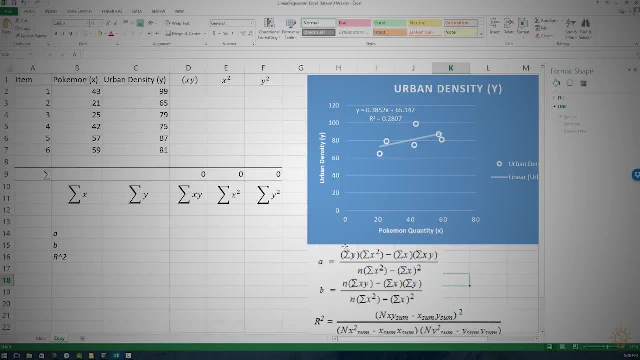 So this is the equation that we have, And that over there is the sum of y- You can find it over there. Then you have the sum of x squared, which is over here, And the sum of x Over there, And the sum of x times y. 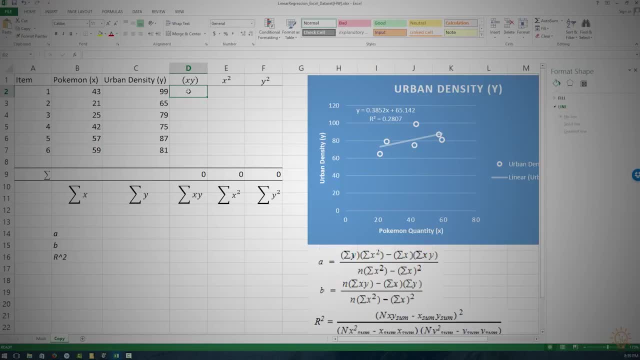 And n is the number of items in our dataset. So first we calculate x times y, And we can take 59 times 81. And this is our answer, And then we can just spread it across And then we've got our product of x and y. 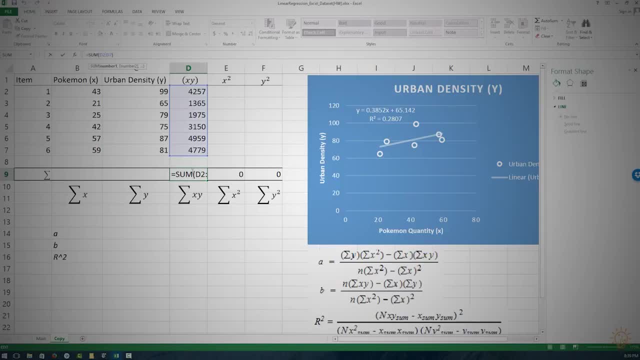 We can create the sum of that, So then that will give us sum of x times y. And then we can do the same for our data set, And then we can create the sum of that, So then that will give us sum of x times y. 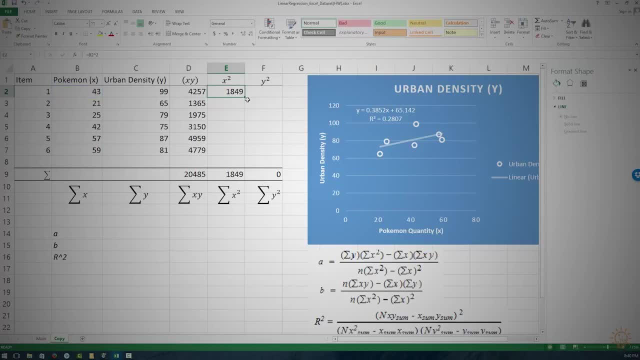 And then we can do the same for our data set, And then we take the X squared, And then we take the squared of 43.. We can do the same for the rest of our data set, And the same we can do for y. 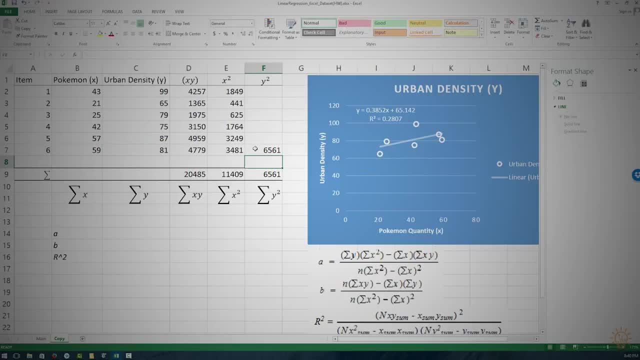 So we take y times itself, Get 6,561. And then we have the sum already. Now we can do the same for pokemon. The sum of pokemon quantity As well as the urban density, That will give us the sum of each of our features.